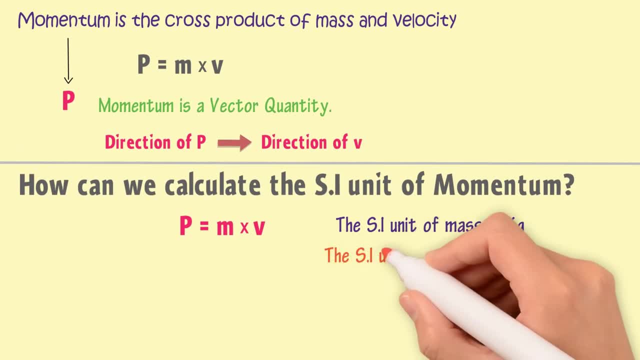 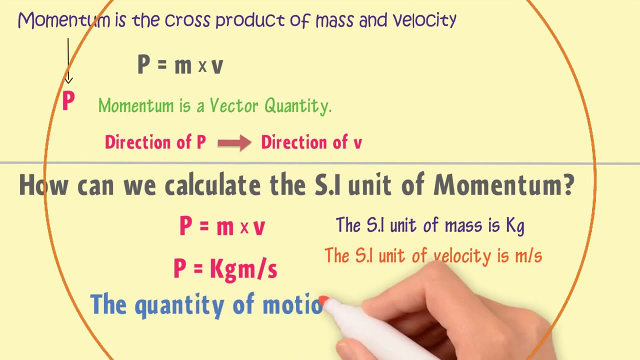 The SI unit of mass is kg and the SI unit of velocity is meter per second. Hence the SI unit of momentum is kg, meter per second. This unit of momentum tells us just the quantity of a motion present in a body or an object. 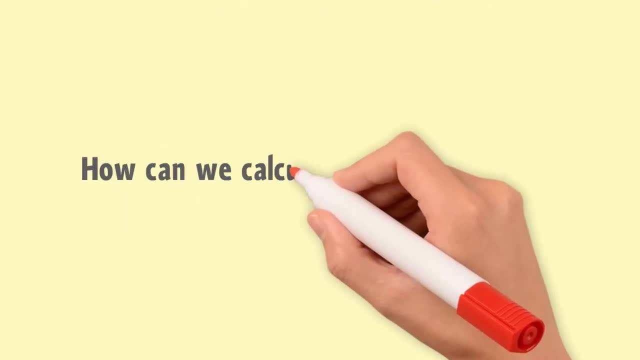 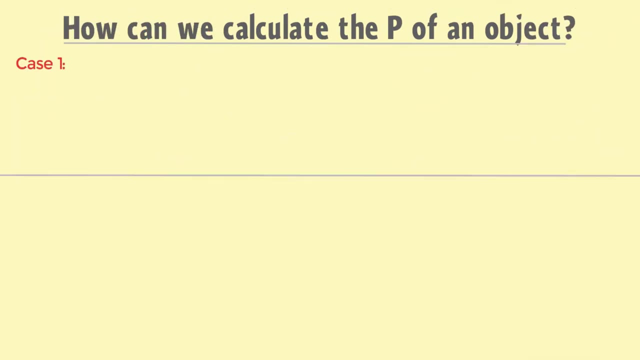 Hence, the SI unit of momentum tells us just the quantity of a motion present in a body or an object. Now, how can we calculate the momentum of an object? Let me give you two cases. In case 1, if a person is standing on a road. 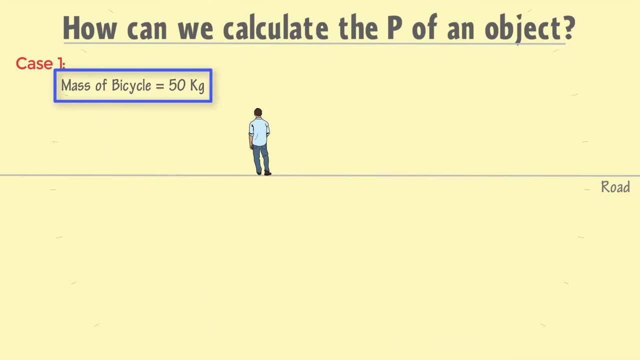 suddenly a bicycle of mass 50 kg, moving with a velocity of 60 meter per second hits the person. As a common observation: the person would only be injured. As a common observation: the person would only be injured. Now consider the same person in case 2.. 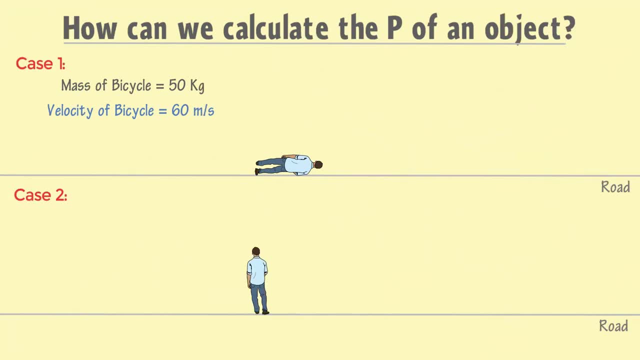 If this person is standing on a road now, suddenly a truck of 2500 kg moving with the same velocity of 60 m per second hits the person. As a common observation: the person may die. Can you guess that a person in case 1 is only or merely injured, while the person in case 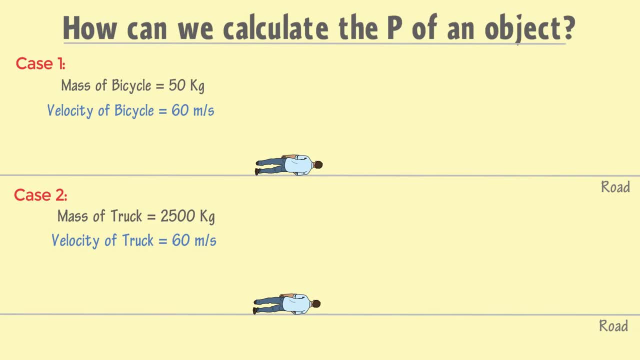 2 is either died or in serious condition, Although both the bicycle and truck were moving with the same velocity- of 60 m per second. I hope that your answer would be the difference in masses. If it is so, then you are 100% right. 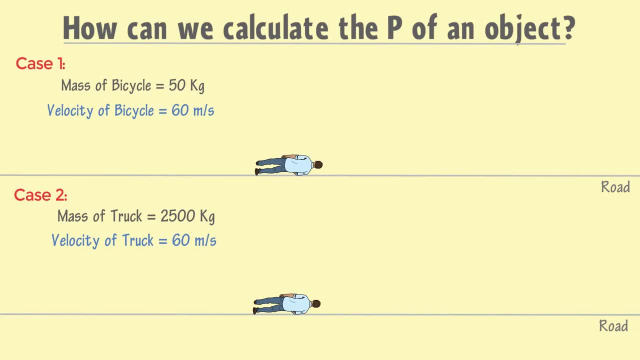 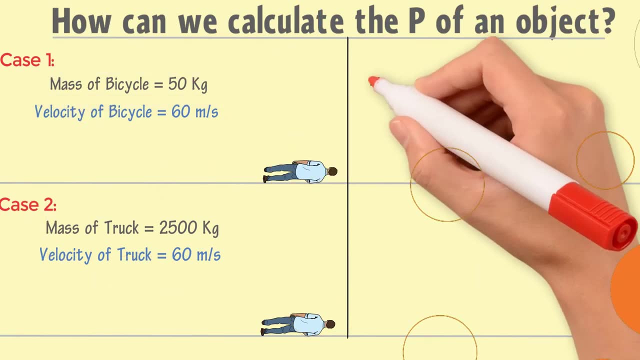 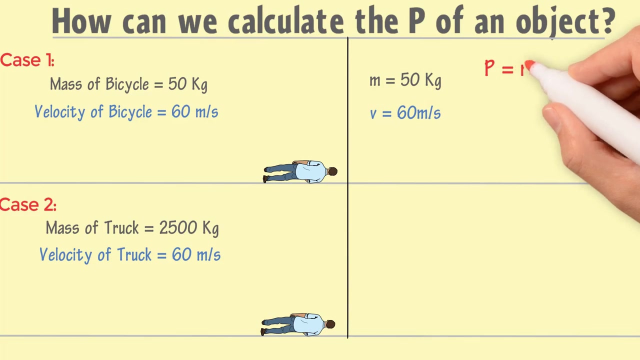 Let me explain these two. In case 1, the mass of the bicycle is 50 kg. It means mass is equal to 50 kg and its velocity V is equal to 60 m per second. Hence the momentum P of the bicycle is equal to mass of the bicycle and the velocity of 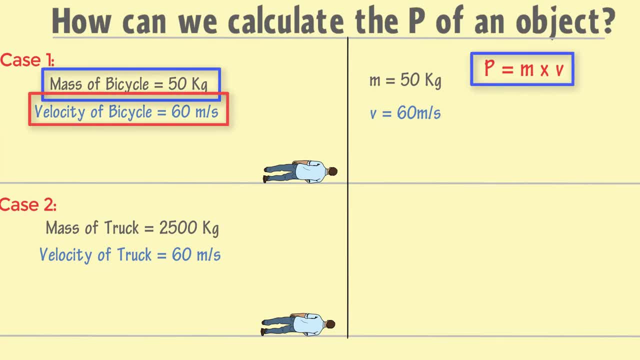 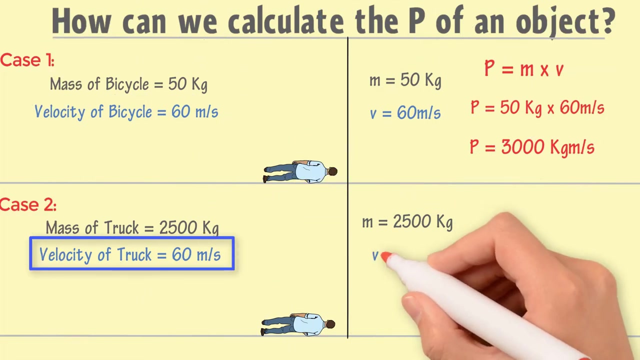 the bicycle Now putting values in the formula P is equal to 50 kg and to 60 m per second, We get 3000 kg m per second. Hence the momentum of bicycle is 3000 kg m per second. In case 2, the mass of the truck, M is equal to 2500 kg, while the velocity of the truck 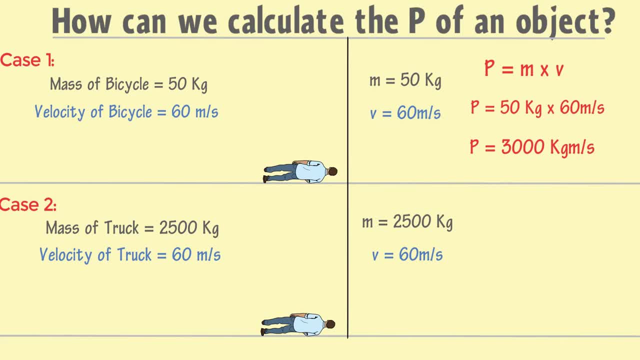 is 60 m per second. Hence the momentum of bicycle P is equal to mass of the bicycle and to velocity of the bicycle. Thus P is equal to 2500 kg and to 60 m per second. We get P is equal to 150000 kg m per second. 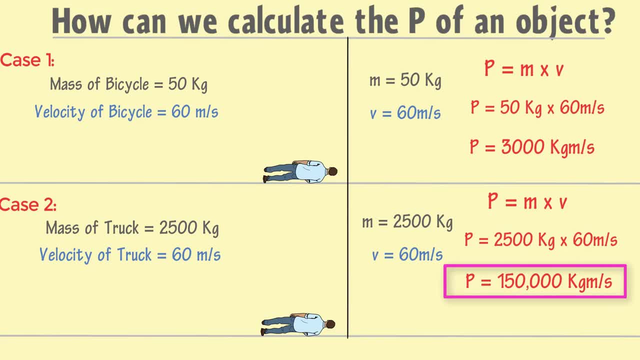 So the momentum of bicycle is 150000 kg m per second. Hence the mass of the bicycle is 20000 kg m per second. kg meter per second. This shows that the momentum of a bicycle is smaller than that of the momentum of a truck. Therefore, a person is merely injured in case 1 when it was hit by the bicycle. 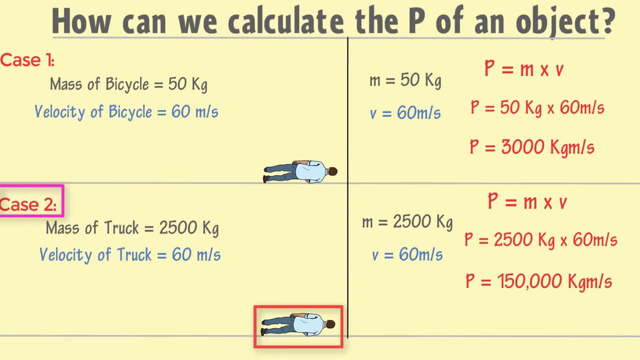 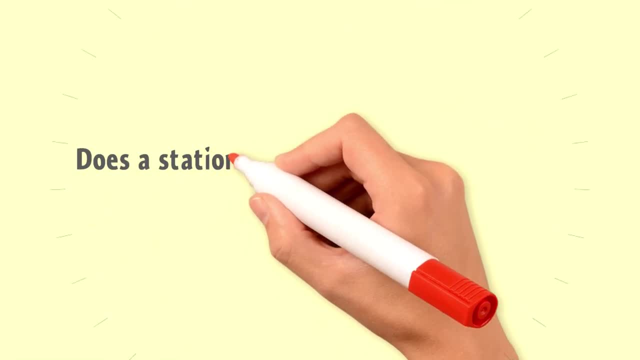 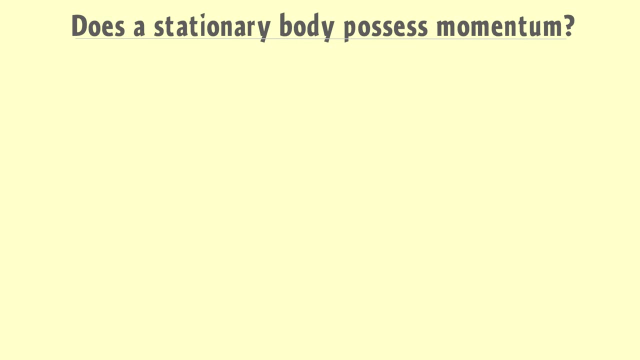 while in case 2, the person got serious injuries or death when it was hit by the truck. At last, let me teach you. does a stationary body possess momentum? To answer this question, let me give you another example. If a car of mass m is stationary or at rest, 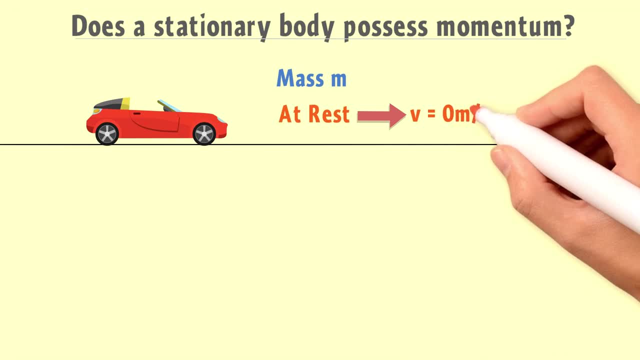 its velocity v is equal to 0 meter per second, Hence its momentum is equal to. p is equal to m to v. Thus p is equal to 0 meter per second, Hence its momentum is equal to. p is equal to m. 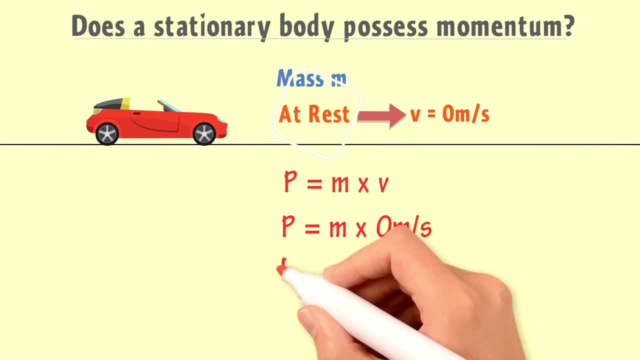 to v. Thus p is equal to m to v, Hence p is equal to m to v. Hence p is equal to m, to v, equal to m and to zero, or p is equal to zero kg meter per second. It shows that if an object is 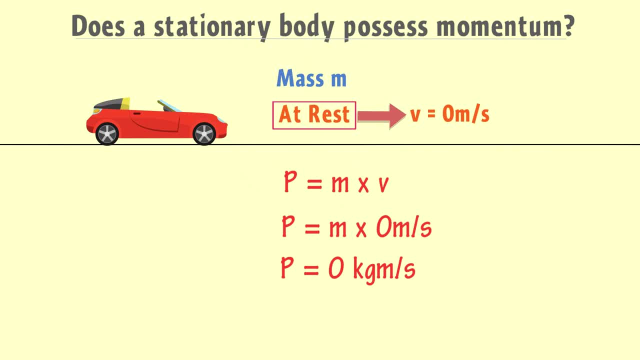 at rest, its momentum p would be zero. or we can say that the momentum p of an object would be zero if the body is at rest. I hope you have learned the fundamental concept of momentum. Thank you very much for watching this video.